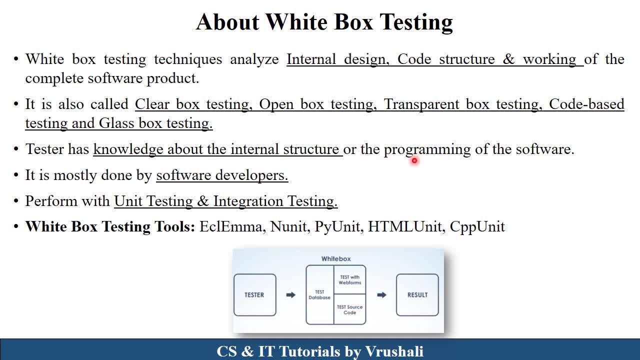 box testing tester require A complete knowledge of programming language and internal structure of your product. White box testing generally performed by the software developer. They write different types of test cases for testing all the internal structure of your project. White box testing performed with unit and integration testing. We will discuss unit and integration testing in detail. 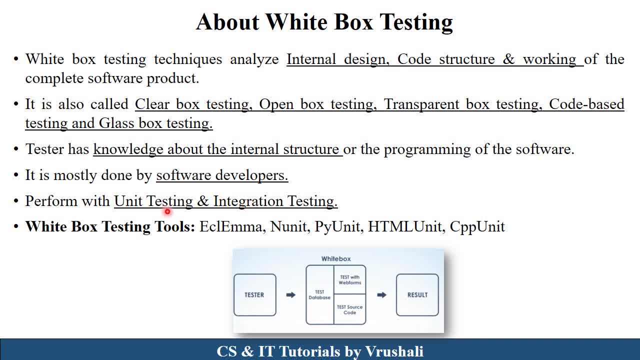 in next session. But here unit testing means to test a module by module, complete your project. And integration testing means to test complete product at the same time. Now there are different white box testing tools are available in market. Tester. use this tools for testing a particular 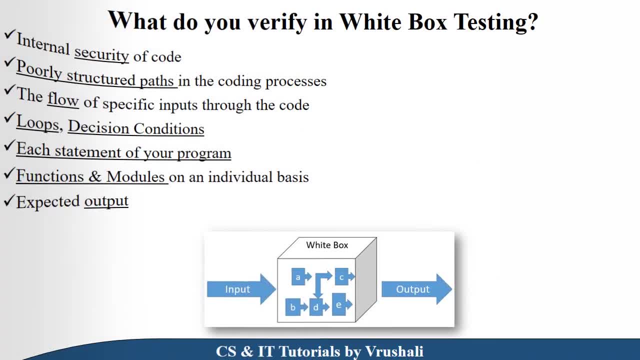 internal structure of your project. Now the next thing is: what do you verify in white box testing? In white box testing tester check that a complete internal security of your code. They check that complete flow of your program from start to end, And they check. 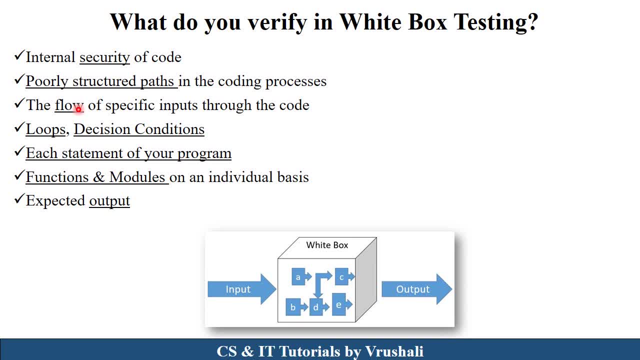 whether it generate a proper output as per the customer requirement or not. Basically, they check the expected output. In your program you have to mention different loops like while loop for loop, Then decision conditions like if else. So they check everything. Tester also check each statement, each and every line mentioned in your program. They also check. 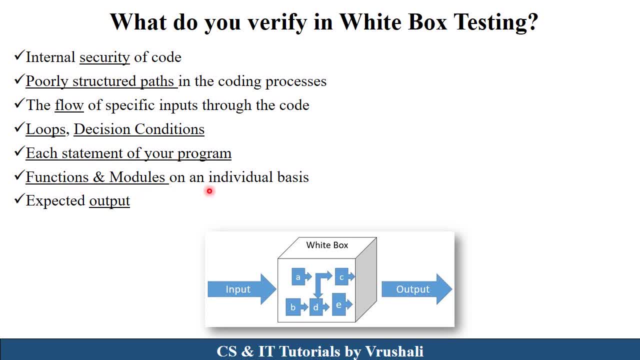 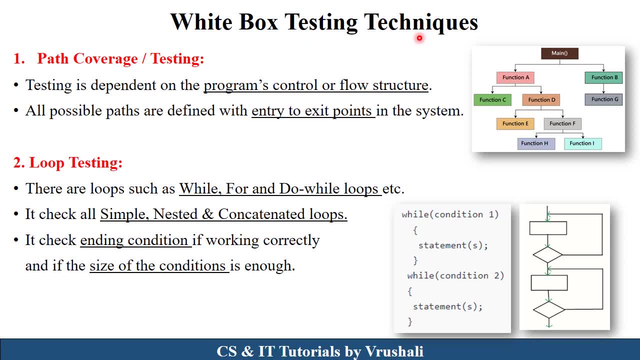 different functions and modules mentioned in your program, your project, on an individual basis. Now Now, Next point is white box testing techniques. The first technique is path coverage or path testing. Here tester check that the complete control or flow of your program, For example, 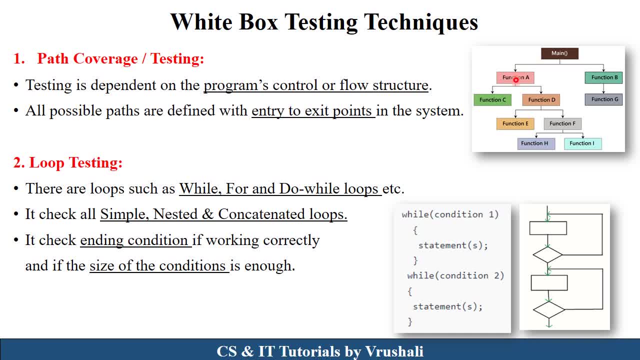 suppose in your program in main function you have to declare function a and function b. From function a you call function c and function d. Now from function d you call function e and function f. So basically they check the complete flow of your program. 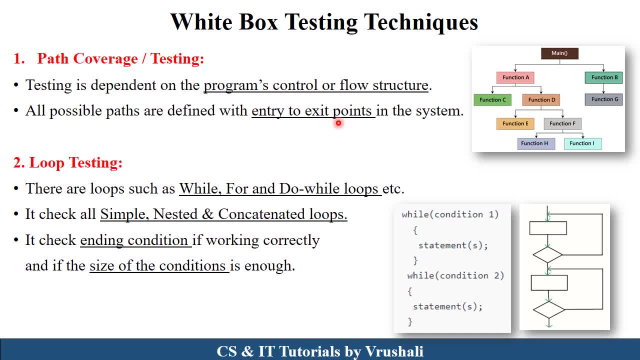 They check entry and exit point of each and every functions and the modules. The next technique is loop testing. So in your program you have to mention different simple, nested and Concatenated loops as per the requirement. So basically, tester, check that while loop for loop. do while loops in your program.